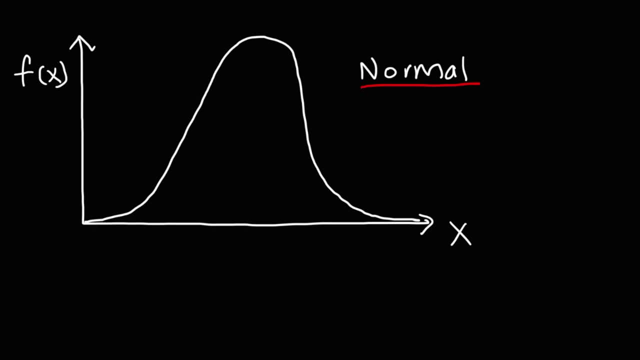 we have the function f of x, which is also known as the pdf, which stands for the probability density function. Now, f of x will tell us the height of the curve above the x-axis at some point x. So f of x will give us the distance between these two points. 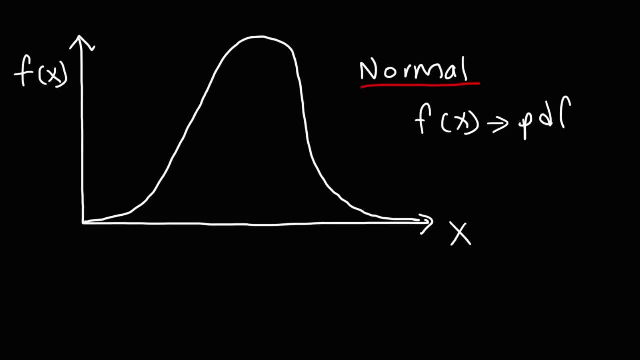 Now let's put some letters here. Let's call this a, b, c and d. We're going to use that shortly, but one thing I do want to mention is that the total area under the curve for a continuous probability distribution is always equal to 1.. 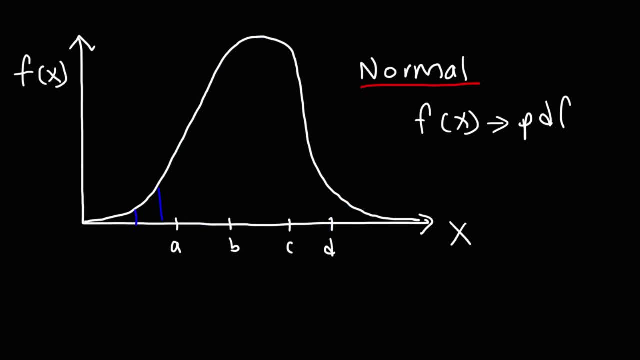 So the area of the shaded region highlighted here In blue, that's equal to 1.. So I'm going to write t a for total area, That's 1.. Let's say, if we wish to calculate the probability that x is less than a. 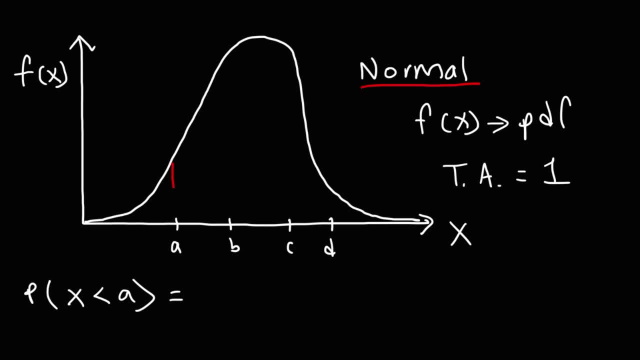 How would you do it? What you need to do is calculate the area under the curve of everything to the left of a, So it's going to be the area of the region shaded in red. Likewise, if we wish to calculate the probability that x is between b and c, 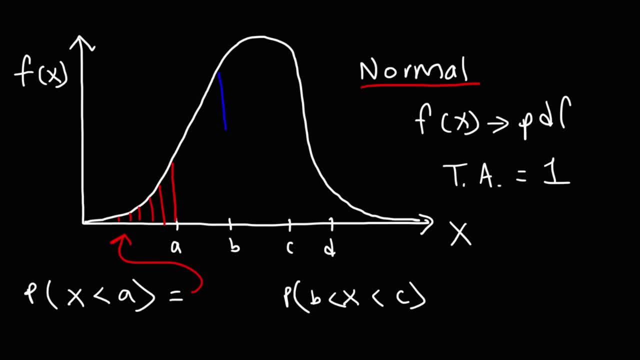 what we need to do is we need to determine the area under the curve between b and c. Likewise, if we wish to calculate the probability that x is greater than d, we need to calculate the area under the curve between b and c. So we're going to calculate the area under the curve to the right of d. 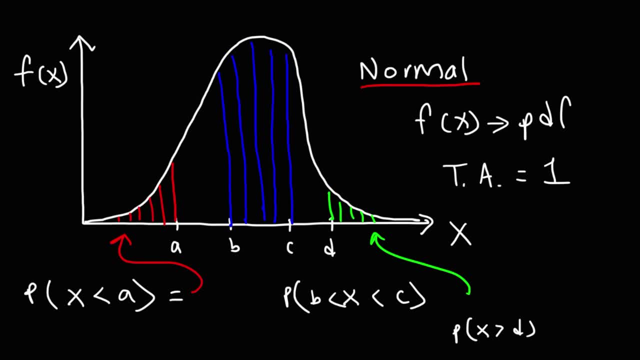 So the probability is always equal to the area under the curve when dealing with a continuous probability distribution function. And keep in mind that f of x is always positive. It's greater than or equal to 0 for all x. So for a continuous probability distribution, you won't see the curve under the x-axis. 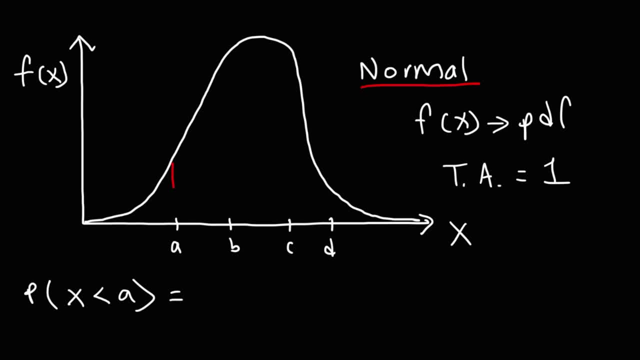 How would you do it? What you need to do is calculate the area under the curve of everything to the left of A, So it's going to be the area of the region shaded in red. Likewise, if we wish to calculate the probability that X is between B and C, 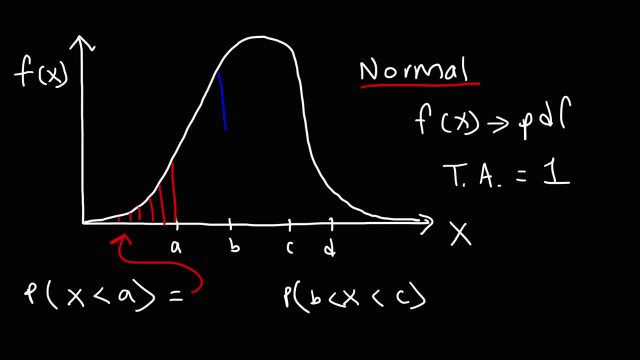 what we need to do is we need to determine the area under the curve between B and C. Likewise, if we wish to calculate the probability that X is greater than D, we need to calculate the area under the curve between B and C. We need to calculate the area under the curve to the right of D. 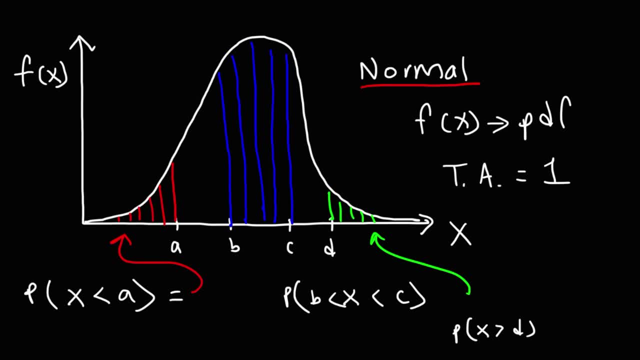 So the probability is always equal to the area under the curve when dealing with a continuous probability distribution function. And keep in mind that F of X is always positive. It's greater than or equal to 0 for all X. So for a continuous probability distribution, you won't see the curve under the X axis. 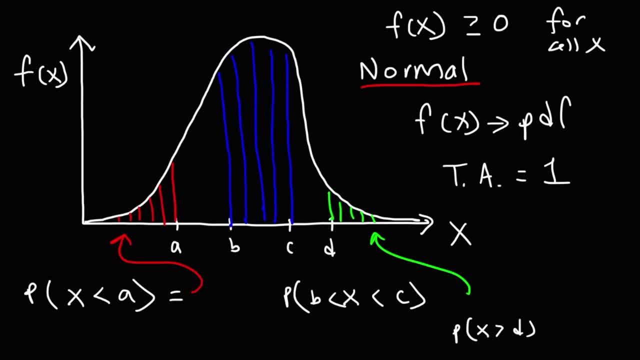 It's always above the X axis. It's always below the X axis. Now here's a question for you: What is the probability that X is equal to B? What would you say? Now, here we don't have a range of values. 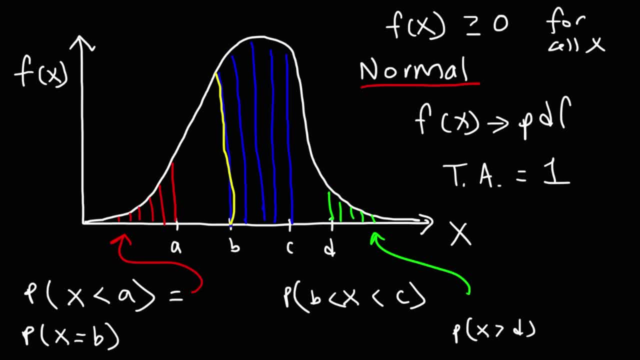 We simply have just a line at B, And for a line like that, the area is 0 because there's no width. You only have height but no width. So you just have to keep in mind that there's no width. So you just have to keep in mind that there's no width. 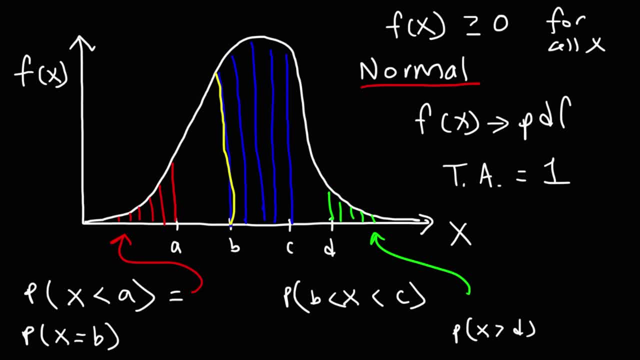 And for a line like that, the area is 0 because there's no width. If you try to calculate the area of a rectangle that only has height but no width, it's nothing. So whenever you try to calculate the area of a finite point, it's going to be 0.. 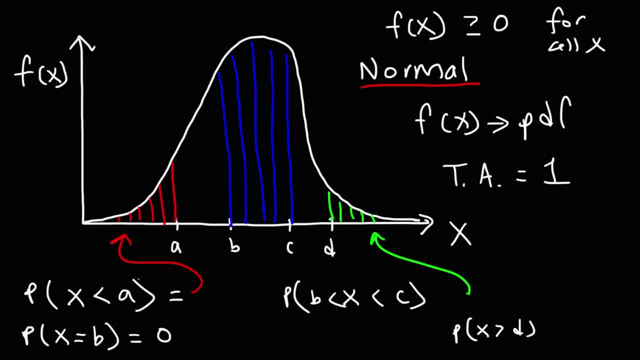 The only way you're going to get a value above 0 is you need to. x has to have a range of values. It can't have a single value. So just keep that in mind. Now, another thing that you want to keep in mind: 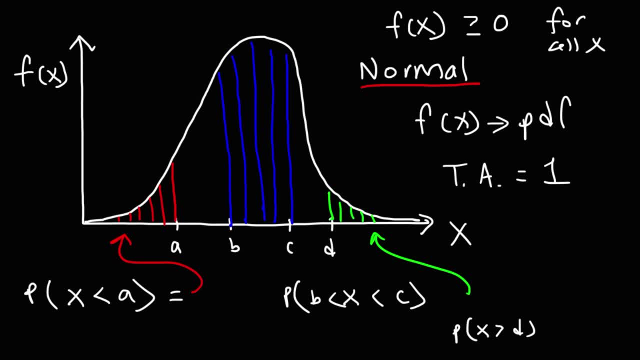 It's always above the x-axis. It's always below the x-axis. Now here's a question for you: What is the probability that x is equal to b? What would you say? Now, here we don't have a range of values. 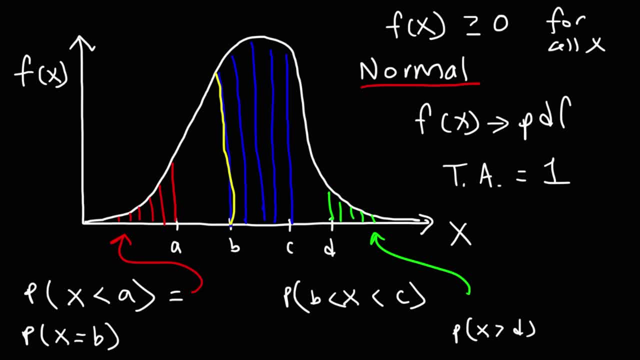 We simply have just a line at b, And for a line like that the area is 0 because there's no width. You only have height, but no width. So you only have height but no width. if you try to calculate the area of a rectangle that only has height but no width, it's nothing. 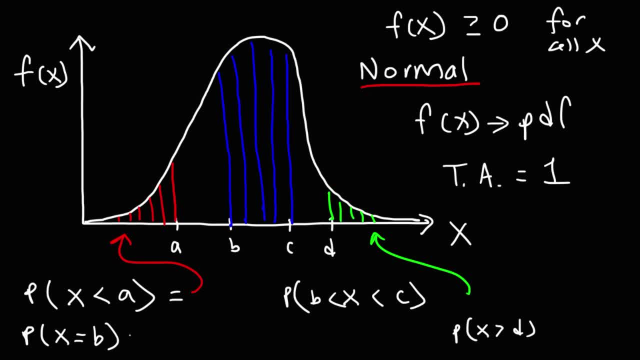 so whenever you try to calculate the area of a finite point, it's going to be zero. the only way you're going to get a value above zero is you need to. x has to have a range of values. it can't have a single value, so just keep that in mind. now, another thing that you want to keep in mind: 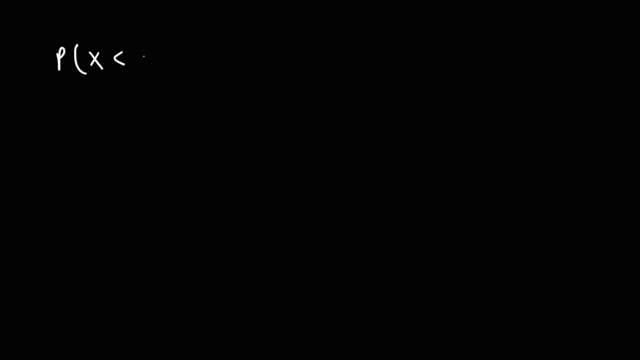 let's say, if you wish to calculate the probability that x is less than a, this is the same as the probability that x is less than or equal to a, because the probability that x is equal to a is zero. so less than or less than and equal to, it's going to be the same. 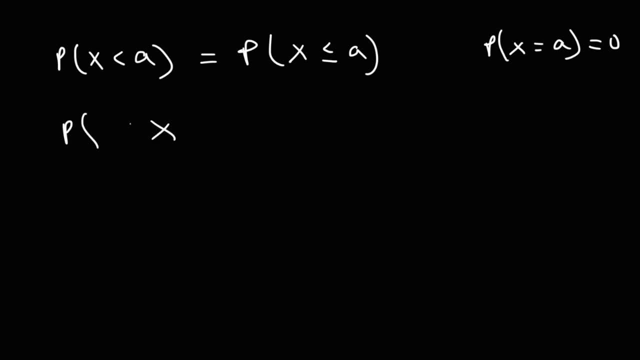 so let's say, if we want to calculate the probability that x is between b and c, this is the same the probability that X is equal to or greater than B, but less than or equal to C. So those are some other things that you want to keep in mind when dealing. 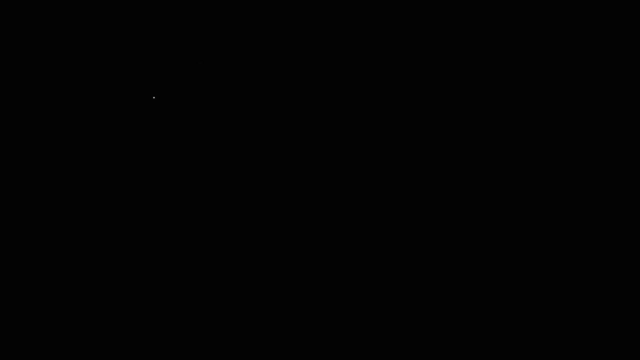 with continuous probability distribution functions. Now we briefly talked about the shape of the normal distribution. There are some other continuous probability distributions you need to be familiar with. The next one is the uniform distribution. The uniform distribution has a constant f of X value, as you can see, and it ranges from A to B. Now the area of the curve under the 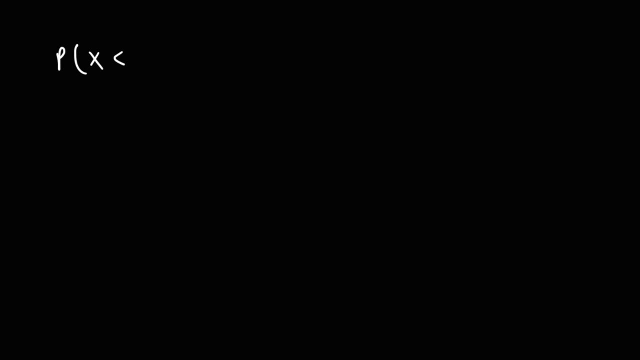 let's say, if you wish to calculate the probability that x is less than a, This is the same as the probability that x is less than or equal to a, Because the probability that x is equal to a is 0.. So less than or less than and equal to, it's going to be the same. 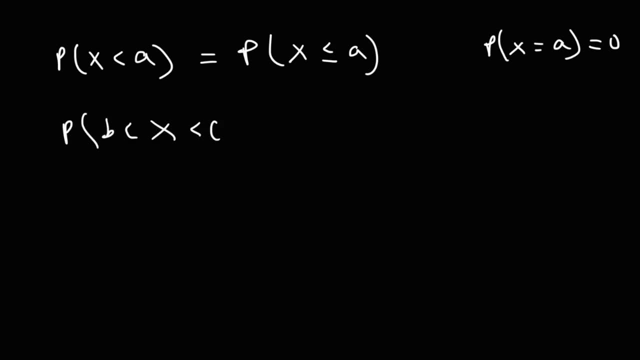 So let's say, if we want to calculate the probability that x is between b and c, this is the same As the probability that x is equal to or greater than b, but less than or equal to c. So those are some other things that you want to keep in mind when dealing with continuous probability distribution functions. 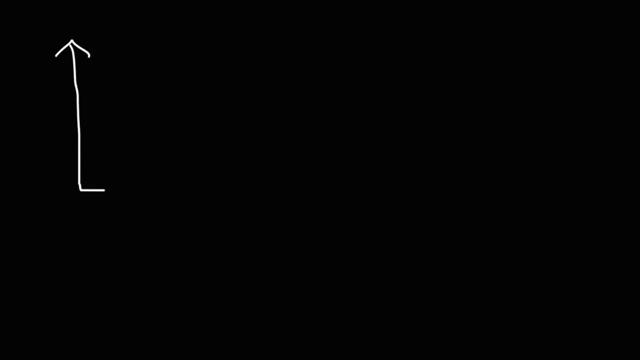 Now we briefly talked about the shape of the normal distribution. There are some other continuous probability distributions you need to be familiar with. The next one is the uniform distribution. The uniform distribution has a constant f of x value, as you can see, And it ranges from a to b. 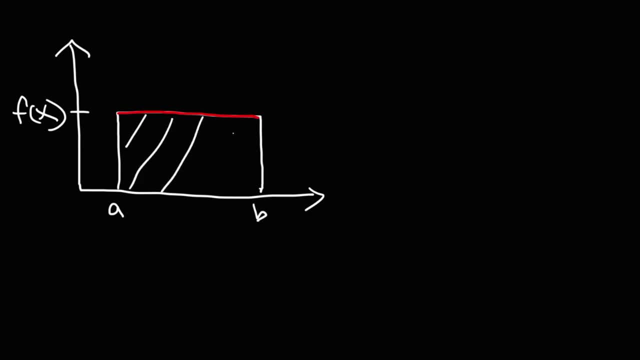 Now the area of the curve under the uniform distribution, or basically the area of the rectangle, is going to be 1.. So let's say we have a uniform distribution from, let's say, 2 to 6.. So a is 2,, b is 6.. 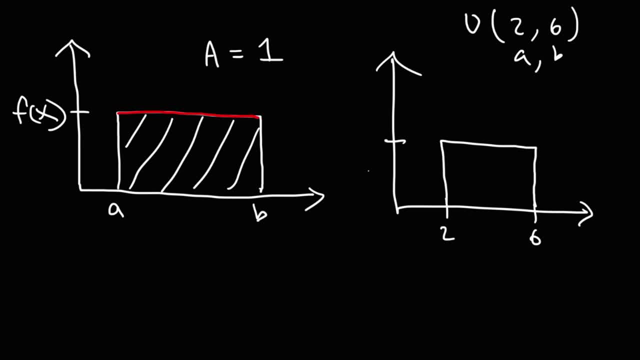 If the area of the rectangle is 1, what is f of x? What is the value that corresponds to that point? Well, we know the base of the rectangle is 4.. 4 times what number is 1?? Because the area has to be 1.. 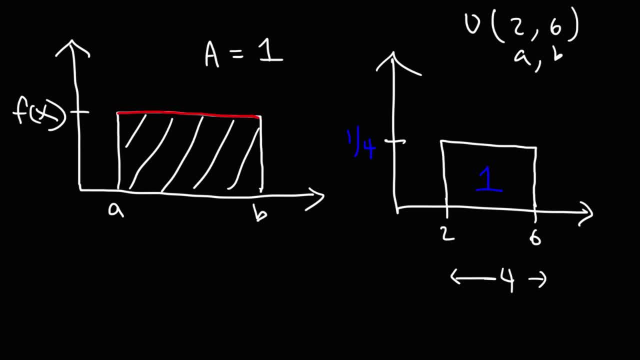 It's going to be 1 over 4.. So that is going to be the value of f of x for this problem for uniform distribution, Because if you multiply 1 fourth by 4, you're going to get an area of 1.. 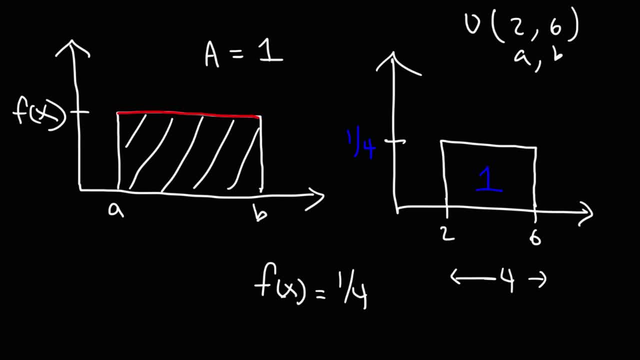 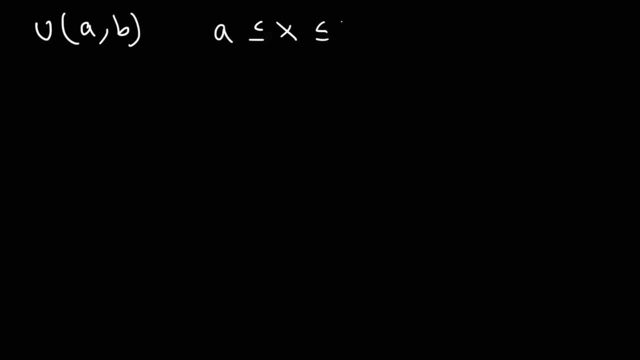 And so for any uniform distribution, the area under the curve has to be 1.. So just keep that in mind. So now I want to give you some formulas that you need to know when dealing with the uniform distribution. So for uniform distribution from a to b, x will vary between a and b. 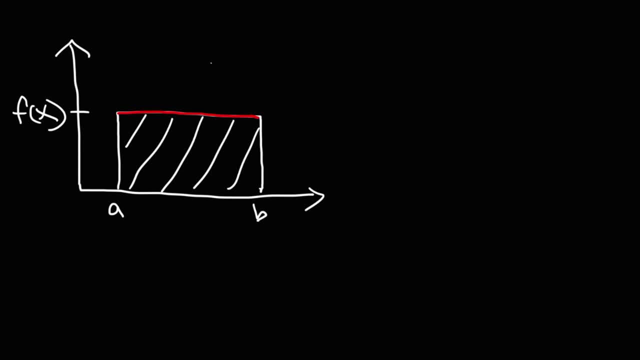 uniform distribution or basically the area of the rectangle is going to be 1.. So let's say we have a uniform distribution from, let's say, 2 to 6.. So A is 2, B is 6.. If the area of the rectangle is 1, what is f of X? 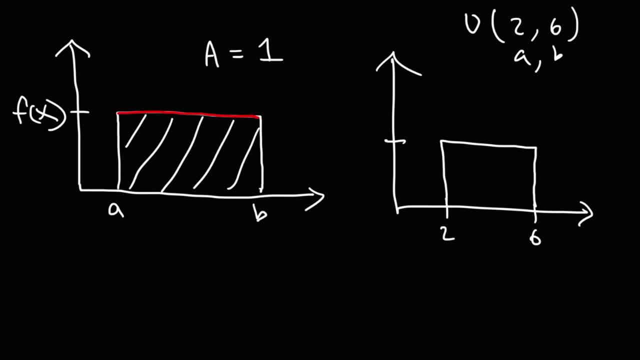 What is the value that corresponds to that point? Well, we know the base of the rectangle is 4.. 4 times what number is 1?? Because the area has to be 1.. It's going to be 1 over 4.. So that is going to be the 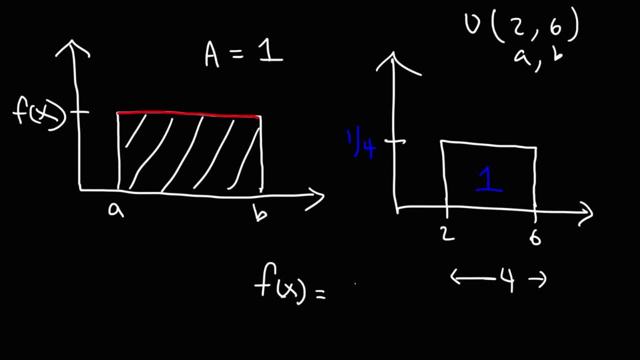 value of f of X for this problem for uniform distribution, Because if you multiply 1 fourth by 4, you're going to get an area of 1.. And so for any uniform distribution, the area under the curve has to be 1.. So just keep that in mind. 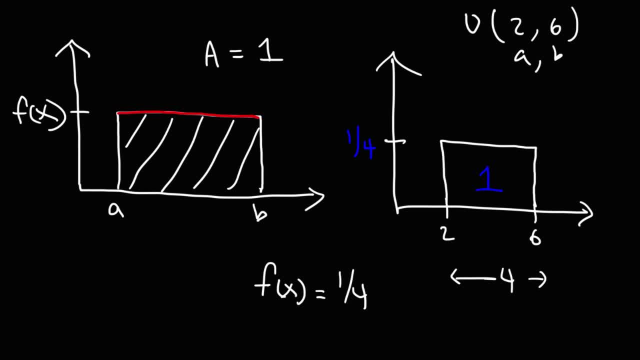 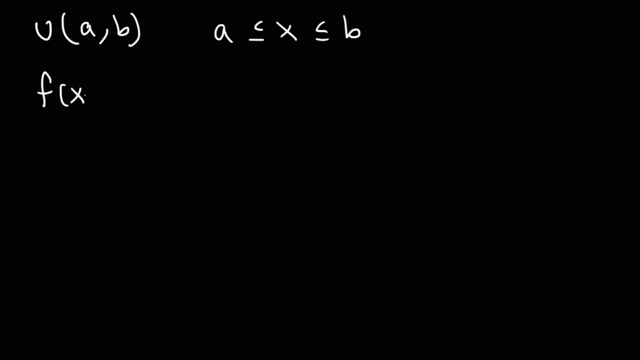 So now I want to give you some formulas that you need to know when dealing with continuous probability distribution functions. So for uniform distribution from A to B, X will vary between A and B. The probability density function f of X is simply 1 over B minus A. 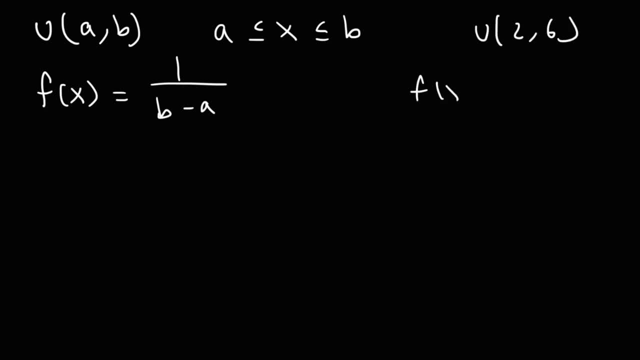 And the last example: if you were to plug in A and B, where B is 6, A is 2,, you would get the function f of X is 6.. Where B is 6, A is 2,, you would get the function f of X is 6.. 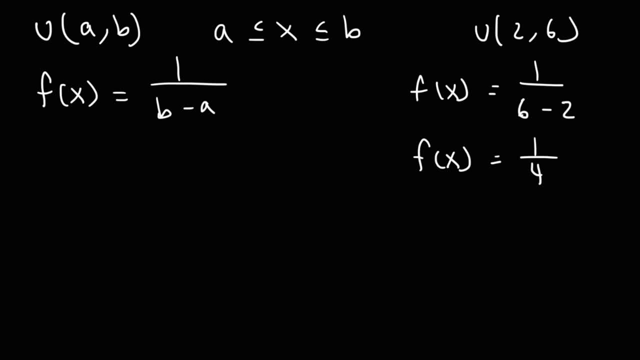 is one over four. So that's how you would incorporate this formula to calculate the probability density function for uniform distribution. Now the next thing you need to know is that the mean is equal to the average of a and b, So it's the sum of a and b divided by 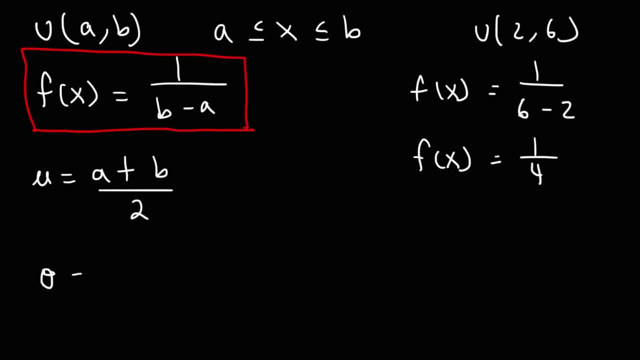 two And x is the standard deviation. That looks like theta but it should be sigma. The standard deviation is the difference between b minus a divided by the square root of 12.. So those are some formulas that you may want to write down when dealing with the uniform distribution, which is one. 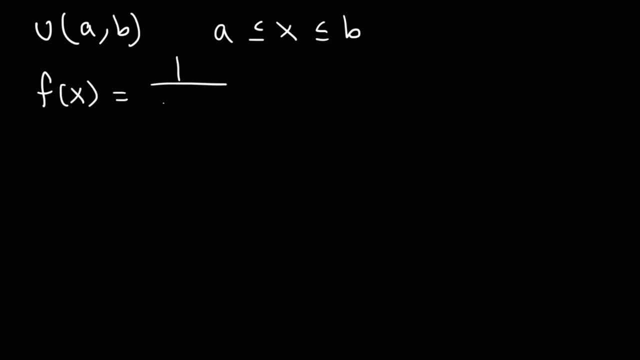 The probability density function f of x is simply 1 over b minus a. In the last example, if you were to plug in a and b, where b is 6, a is 2, you would get the function f of x is 1 over 4.. 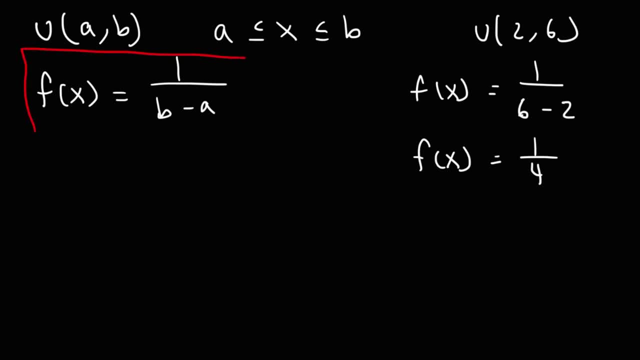 So that's how you would incorporate this formula to calculate the probability density function for uniform distribution. Now the next thing you need to know is that the mean is equal to the average of a and b, So it's the sum of a and b divided by 2.. 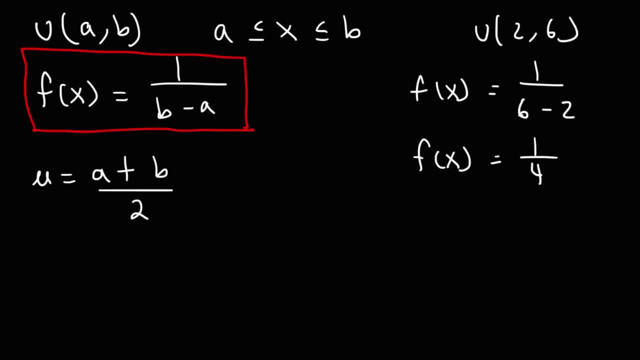 And x is the standard deviation. That looks like theta but it should be sigma. The standard deviation is the difference between b minus a divided by 2. So it's the square root of 12.. So those are some formulas that you may want to write down when dealing with the uniform distribution. 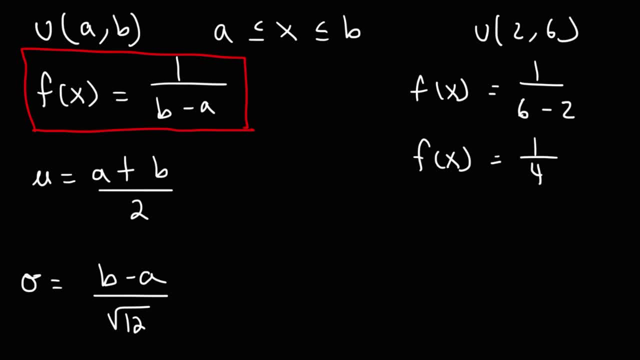 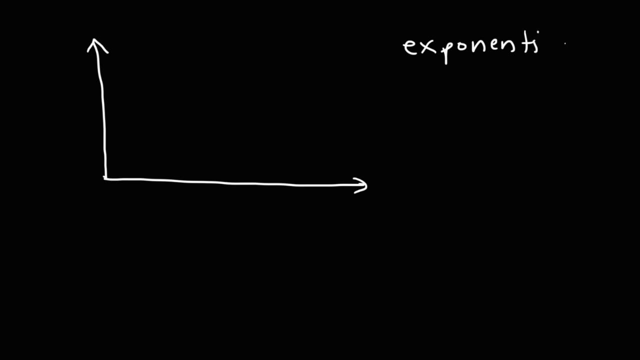 which is one of the types of continuous probability distributions that you need to know Now. the next distribution that we're going to talk about is known as the exponential distribution. This is another continuous probability distribution. This is another continuous probability distribution that you want to add to your list. 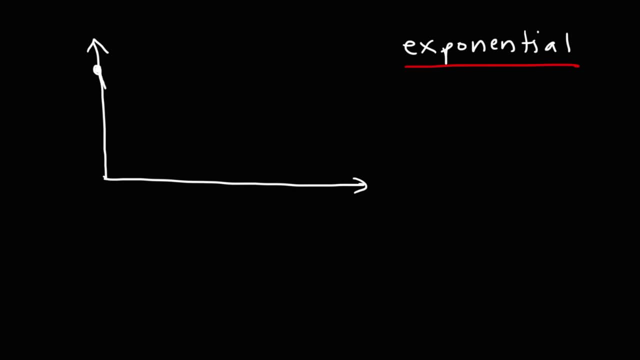 So it has a y-intercept and then the function decreases over time, or with x. We have f of x on the y-axis and the y-intercept is lambda. the rate parameter, The probability density function, is f of x is equal to lambda e. 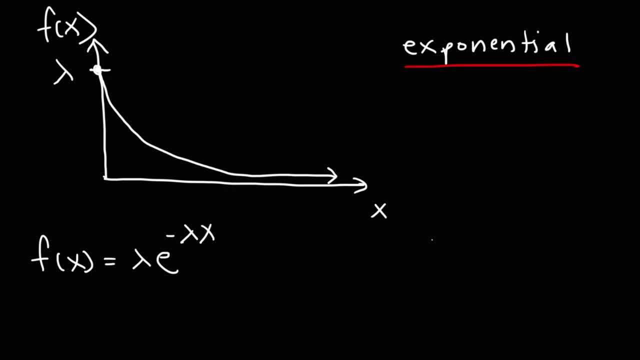 to the negative lambda times x Lambda: the rate parameter is 1 divided by the mean. So those are some things that you want to know for this type of function, And keep in mind the total area under the curve for this one. 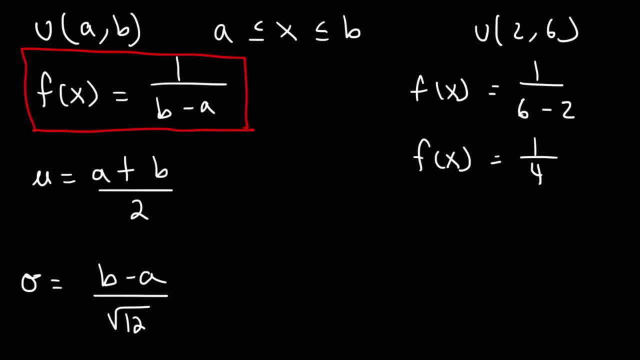 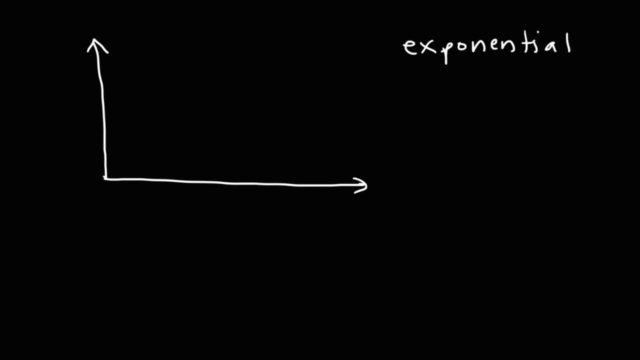 of the types of continuous probability distributions that you need to know Now. the next distribution that we're going to talk about is known as the exponential distribution. This is another continuous probability distribution that you want to add to your list. So it has a y-intercept and then the function decreases over time, or with x. We 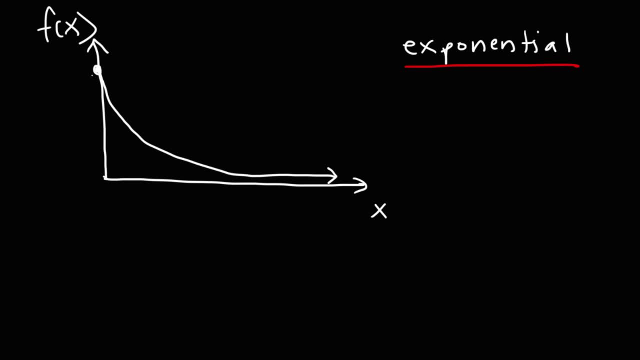 have f of x on the y-axis and the y-intercept is lambda. the rate parameter, The probability density function, is known as the exponential distribution. This is known as the exponential distribution. The function is: f of x is equal to lambda e, to the negative lambda times x. 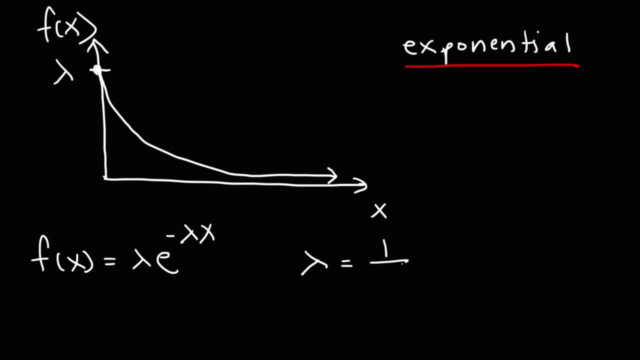 Lambda. the rate parameter is one divided by the mean. So those are some things that you want to know for this type of function. And keep in mind the total area under the curve for this one or any type of continuous probability distribution function is always going to be the same. So the function is: f of x is equal to lambda, e to the negative. 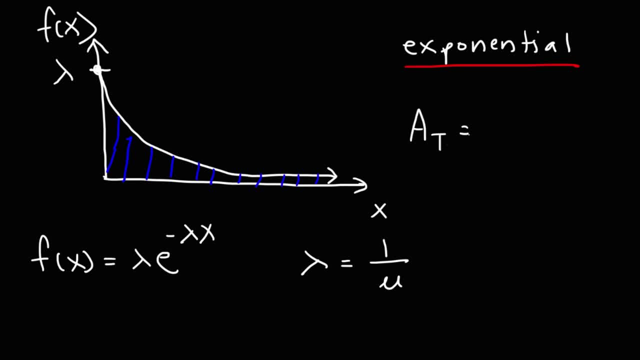 lambda times x. The function is, however, known by all Boolean variables, so it's not defined here. You set f of x as the exponential wealthy, so it's coming from lambda, and then f of y comes from lambda, And so you'll know that your combination of the two Fisherian distributions ultimately 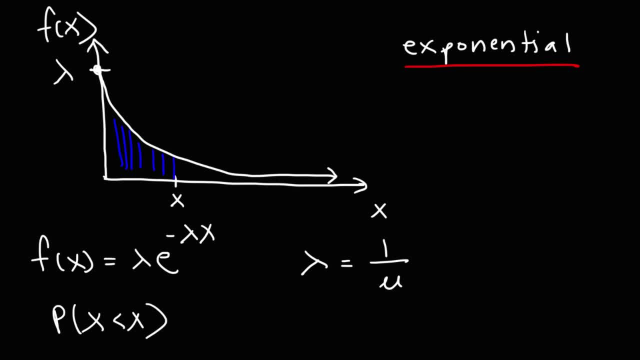 means that you have the argument through the work environment of x prime x to the secondDirectMap remains true. So in case that your particular homem and your other members are having a rough Thursday, then we can simply replace the two work ح approach and go ahead and start over again. If there was a probability of x, then we need to. 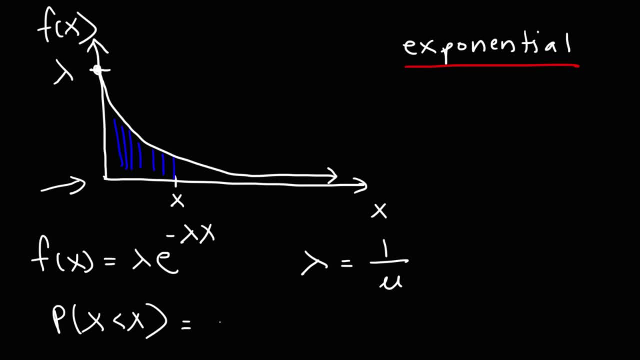 The formula for that? to calculate the area under the curve of that region, it's going to be 1 minus e to the negative lambda times x. Now if we want to calculate the probability that x is greater than x, it's simply e to the negative lambda times x. 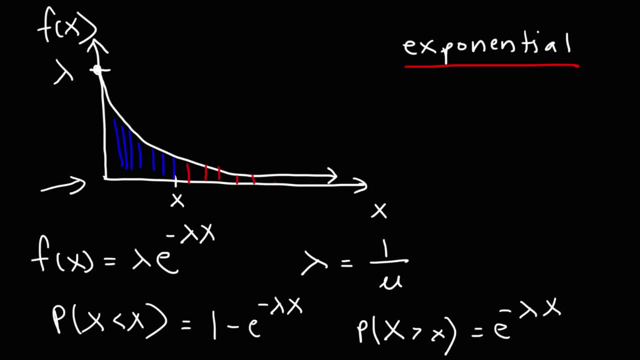 In this case that would represent the region under the curve to the right. So those are some other formulas that you want to know if you need to calculate the probability or the area under the curve.